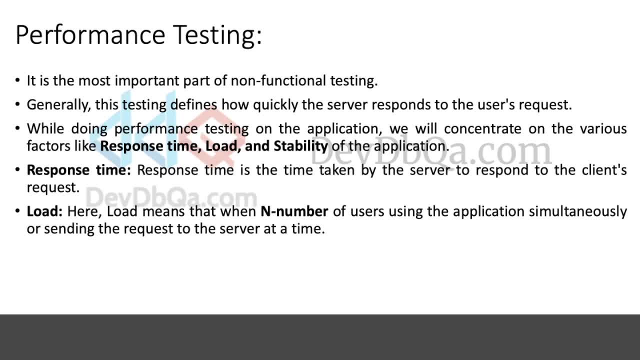 Load Here. load means that when n number of users are using the application simultaneously or sending the request to the server at a time, So the load of the application should be stable, So the application should not crash if n number of users are using the application simultaneously. 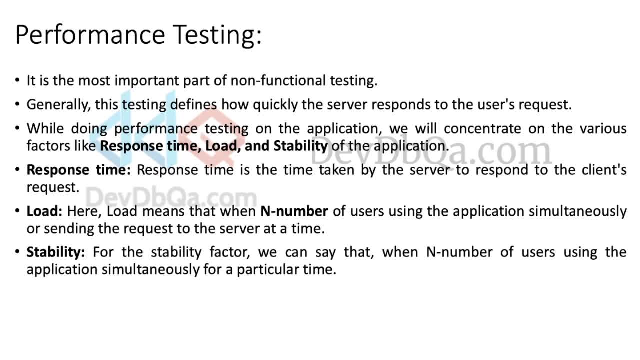 Stability. For the stability factor we can say that when n number of users using the application simultaneously for a particular time. So if a number of users are using the application simultaneously for a particular time, like say for 1 hour or 2 hours, the users are continuously using the application. then the stability 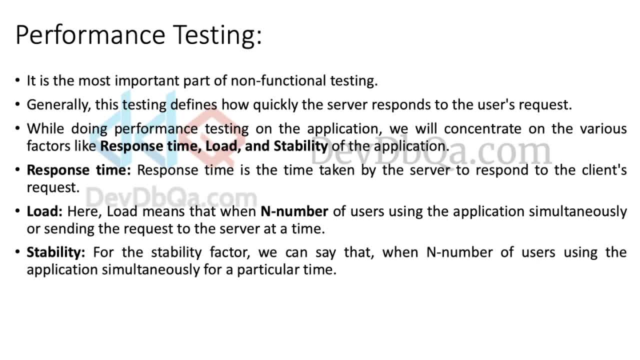 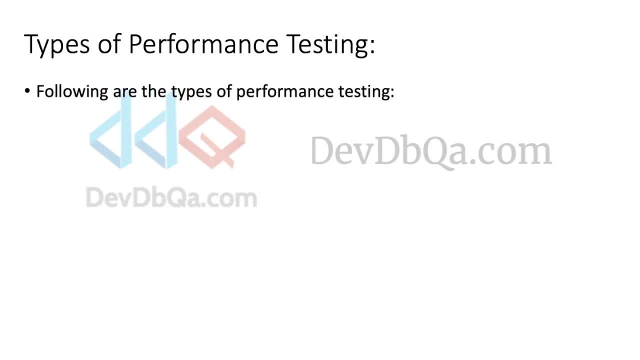 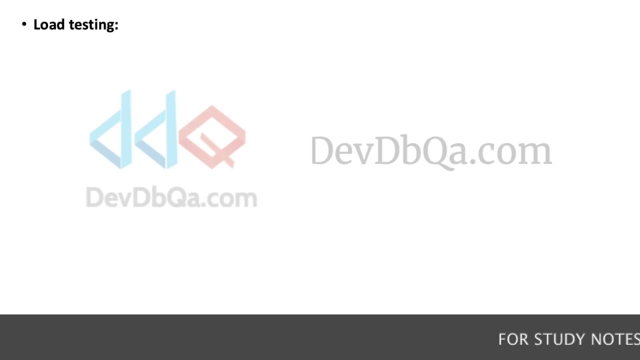 comes in the picture that the application is stable or not. Types of Performance Testing. Following are the types of performance testing: 1. Load Testing, 2. Stress Testing, 3. Scalability Testing. 4. Stability Testing. 1. Load Testing: The load testing is used to check the performance of an application by applying some load which 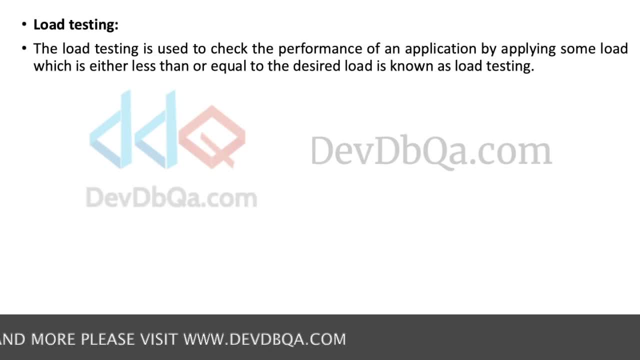 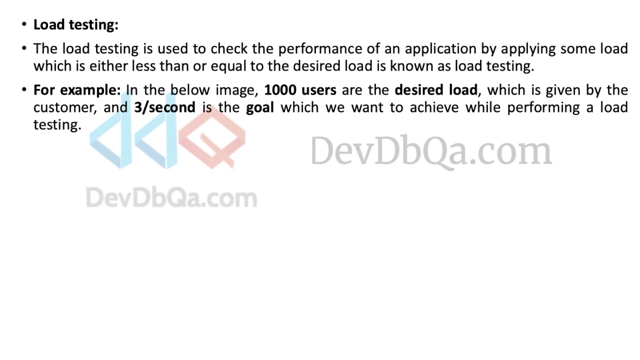 is either less or equal to the desired load is known as load testing. In load testing we apply some type of load on the application, Then check the performance of the application, that the application is behaving properly or not. For example, in this image, 1000 users are the desired load which is given by the customer. 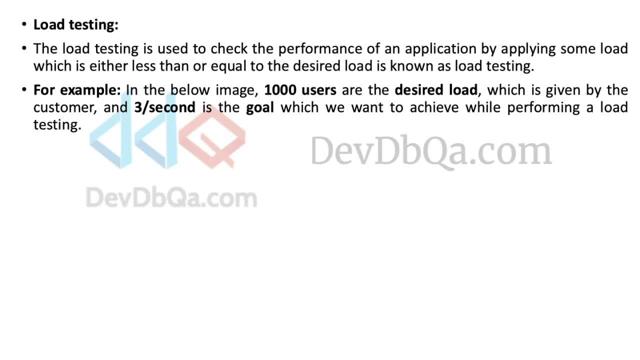 and 3 per second is the goal which we want to achieve while performing a load testing: Stress Testing. The stress testing is testing which checks the behavior of an application By applying load greater than the desired load, for example. if we took the above example, 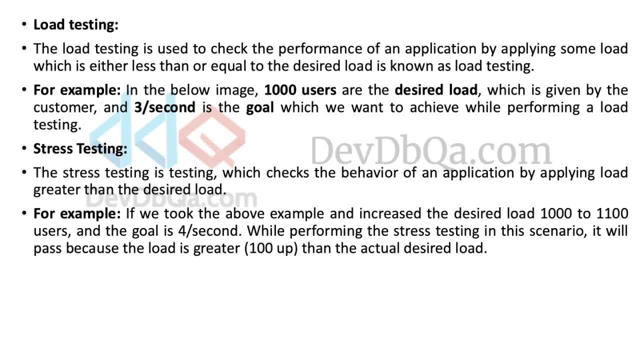 and we increased the desired load from 1000 to 1100 users. the goal is 4 per second While performing the stress testing. in this scenario it will pass because the load is greater than the actual desired load. So in stress testing we check the behavior of the application. 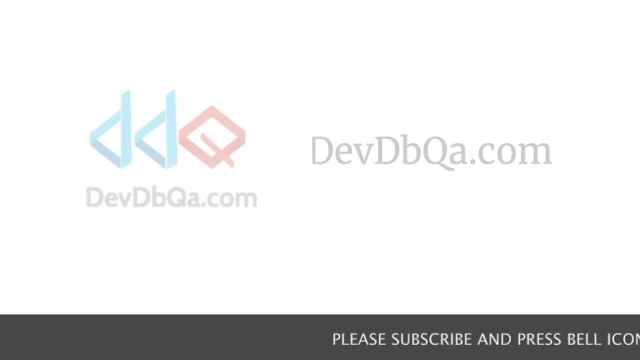 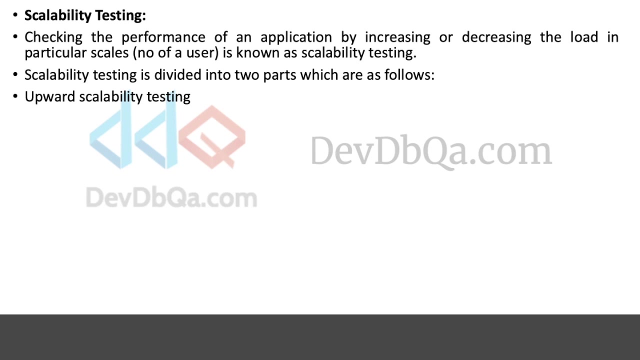 By applying load greater than the desired load Scalability Testing. In scalability testing, checking the performance of an application by increasing or decreasing the load, in particular scales, is known as scalability testing. Scalability testing is divided into two parts, which are as follows: Upward Scalability Testing and Downward Scalability Testing. 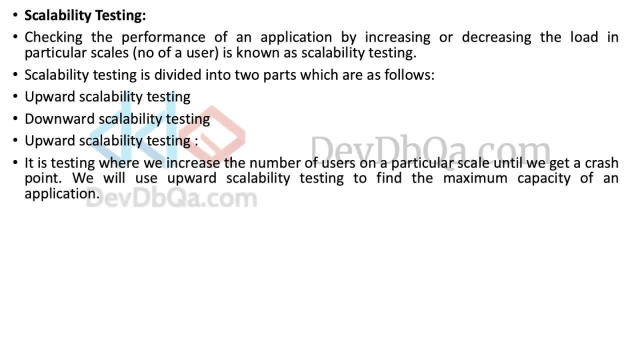 Upward Scalability Testing. Downward Scalability Testing: It is the testing where we increase the number of users on a particular scale until we get a crash point. We will use upward scalability testing to find the maximum capacity of an application. After that point, the application will crash. 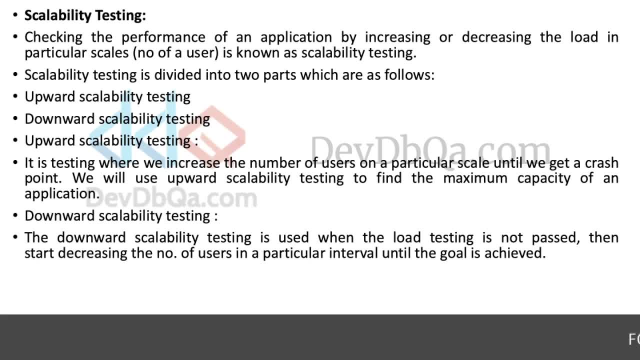 Downward Scalability Testing. Downward Scalability Testing. 2. Upward Scalability Testing. 1. Stability testing is used when the load testing is not passed. then start decreasing the number of users in a particular interval until the goal is achieved. Stability testing: Checking the performance of an application. 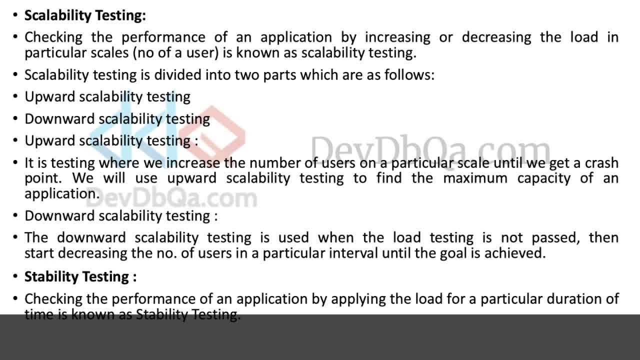 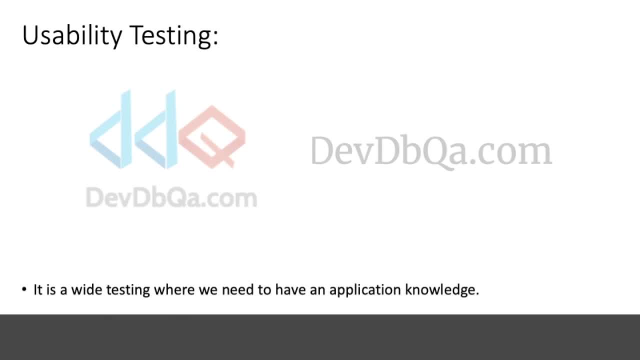 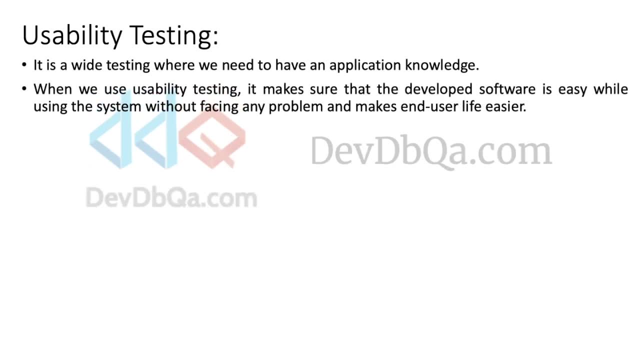 by applying the load for a particular duration of the time is known as stability testing, Usability testing. It is a wide testing where we need to have an application knowledge. When we use usability testing, it makes sure that the developed software is easy while using the system without facing any problem and makes end-user life easier. 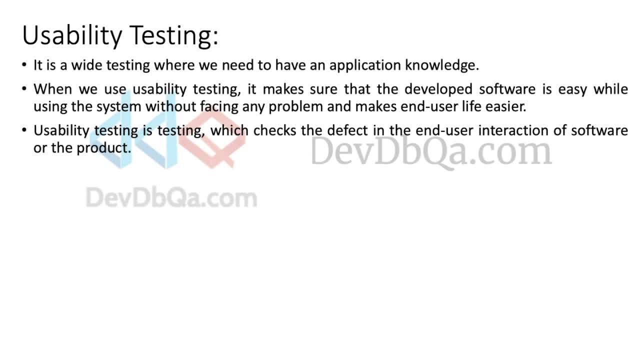 Usability testing is testing which checks the defect in the end-user interaction of software or the product. Usability testing is testing which checks the defect in the end-user interaction of software or the product. It is also known as user experience testing. So usability testing is the testing that the end-user will test that the application is. 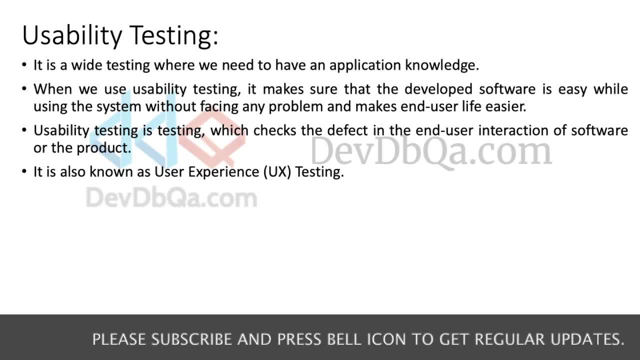 usable or not. The experience of the end-user matters the most in usability testing. User friendliness can be described in many aspects, such as easy to understand, easy to access, look and feel, faster to access, effective navigation and good error detection. 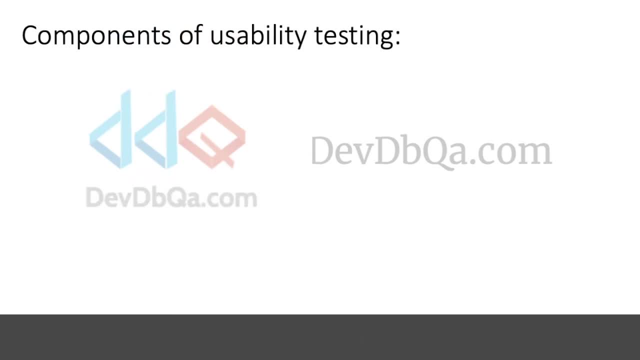 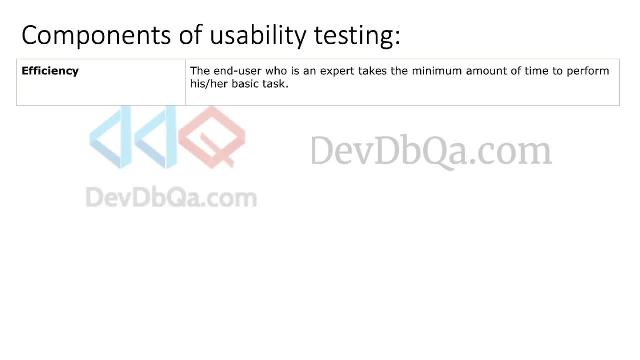 The end-user is the one who will be responsible for the user's handling Components of usability, testing, Efficiency. The end-user, who is an expert, takes the minimum amount of time to perform his or her basic task, So this point is known as efficiency of the application. 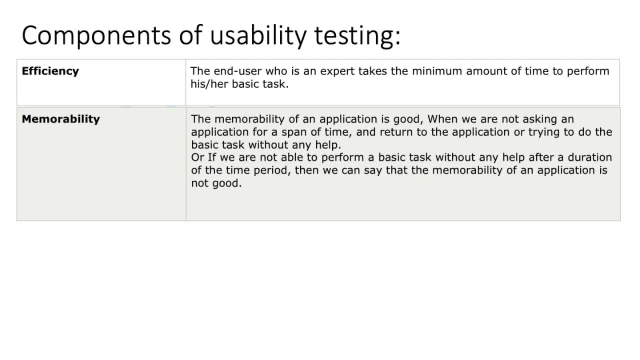 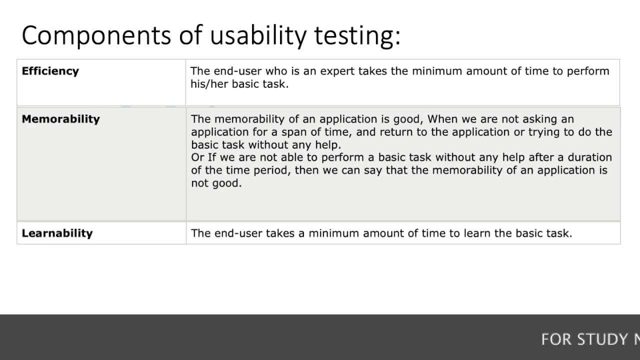 Memorability: The memorability of an application is good when we are not asking an application for a span of time and return to the application, or trying to do the basic task without any help. Learnability: The end-user takes a minimum amount of time to learn the basic task. 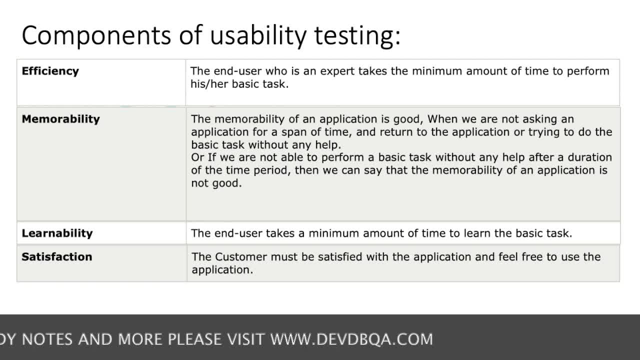 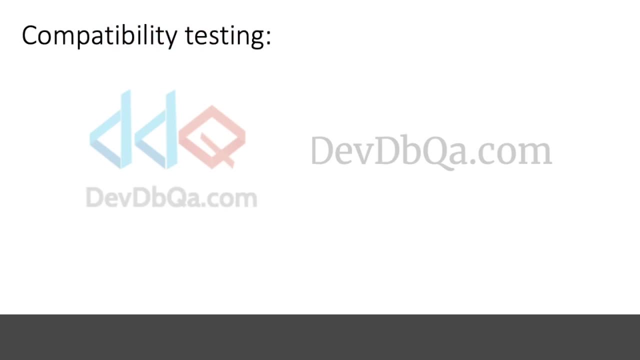 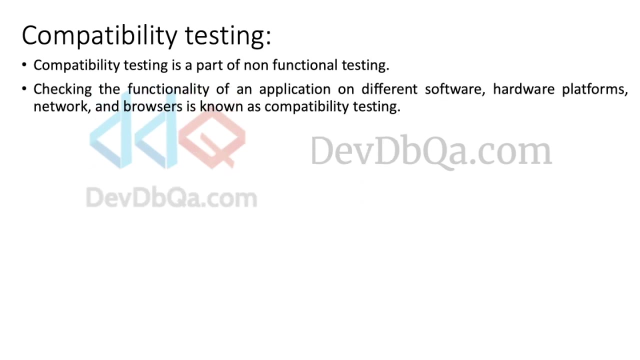 Satisfaction. The customer must be satisfied with the application and feel free to use the application Errors. Here we try to help the end-user to resolve those errors which they made earlier and perform their task again. Compatibility Testing: Compatibility testing is a part of non-functional testing. 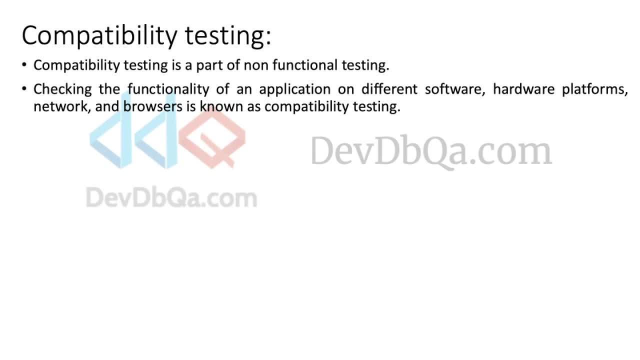 Checking the functionality of an application on different software, hardware platforms, networks and browsers is known as compatibility testing. So in compatibility testing we check that the application is compatible on different types of software, different types of hardware, different types of networks and different 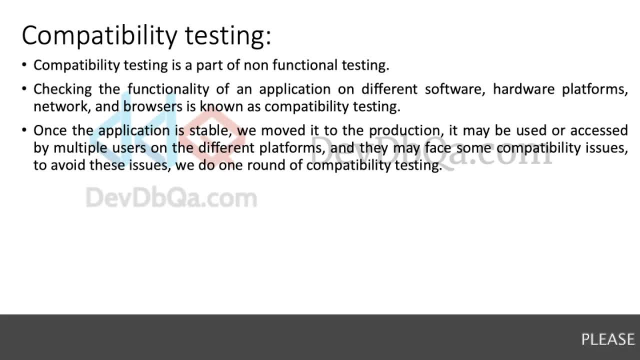 types of browsers, So the application should be compatible with all types of hardware, software and browsers. Once the application is stable, we move it to production. It may be used or accessed by multiple users on the different platforms and they may face 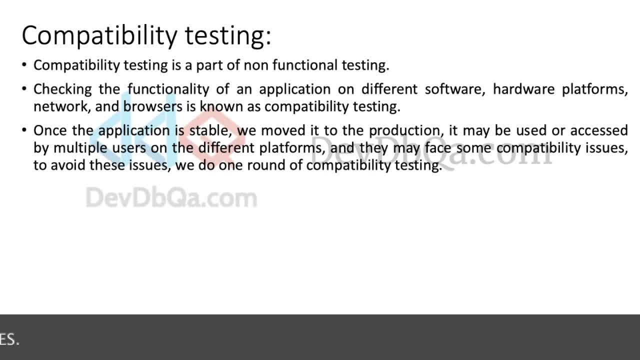 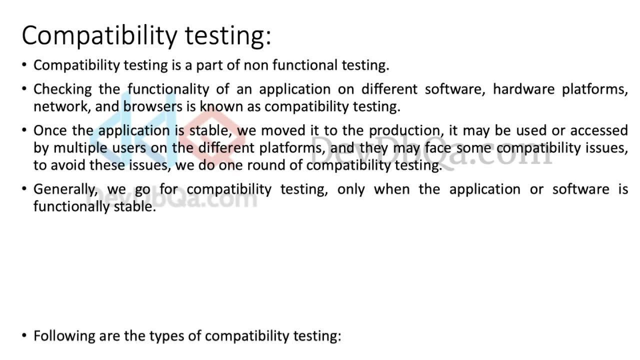 compatibility issues. To avoid these issues, we do one round of compatibility testing. Generally we go for compatibility testing only when the application or software is functionally stable. So the compatibility testing is done only when the software is stable. Following are the types of compatibility testing. 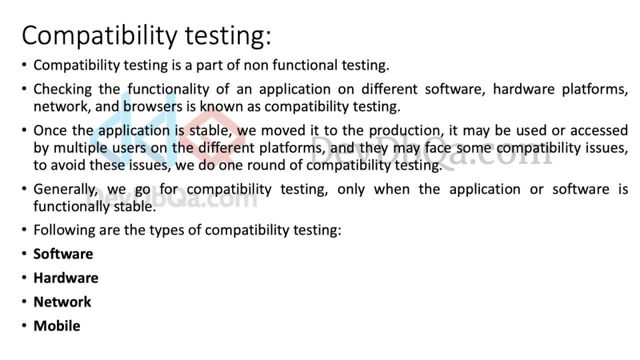 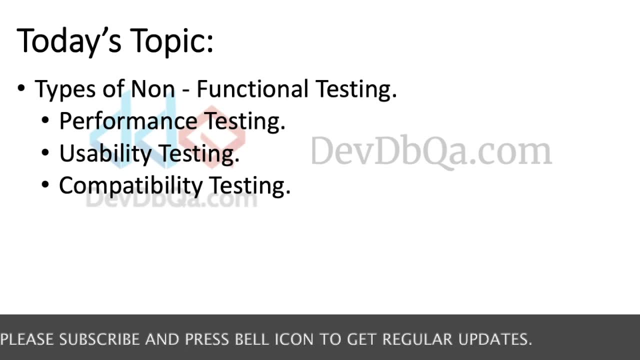 1. Software, 2. Hardware, 3. Network, 4. Mobile. So we test the software on different types of software, different types of hardware, different types of networks and on mobile devices also. So, guys, in today's video we learned about types of non-functional testing that are performance. 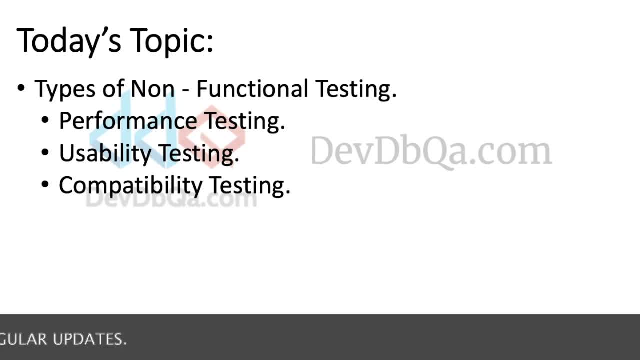 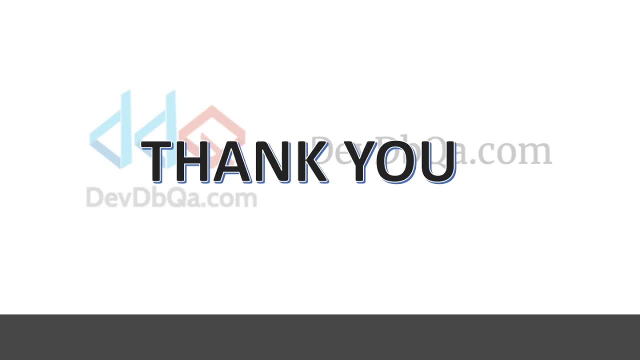 testing, usability testing and compatibility testing. So, guys, if you like my video, then press the like button and please subscribe to my channel to get regular updates. and if you have any suggestions, then please comment in the comment section. Thank you so much. 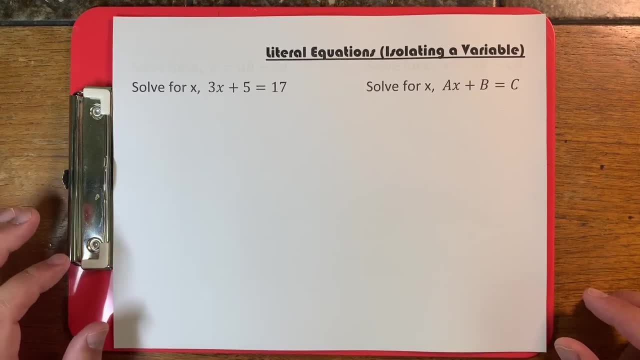 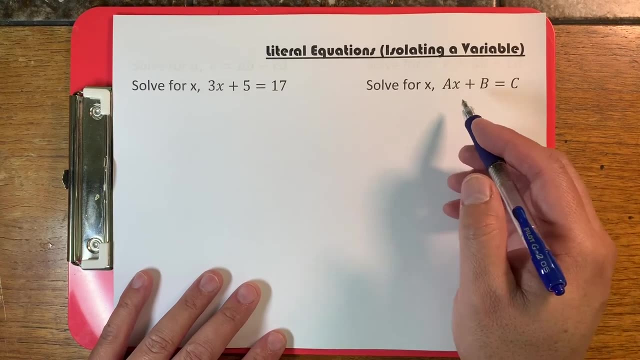 What we're going to work on in this video is how to solve literal equations. Now, what a literally literal equation looks like is something like this, where you have no numbers. What we're asking for is: please solve for x. Now let's look at something that we recognize. 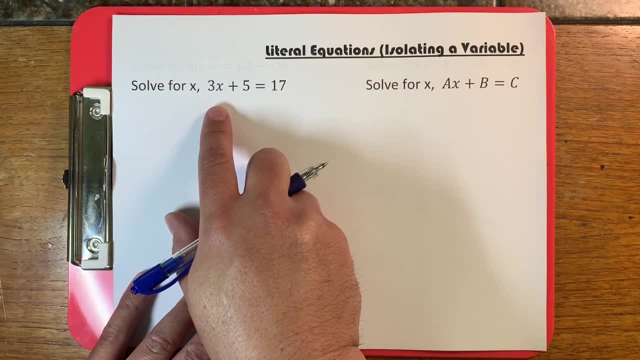 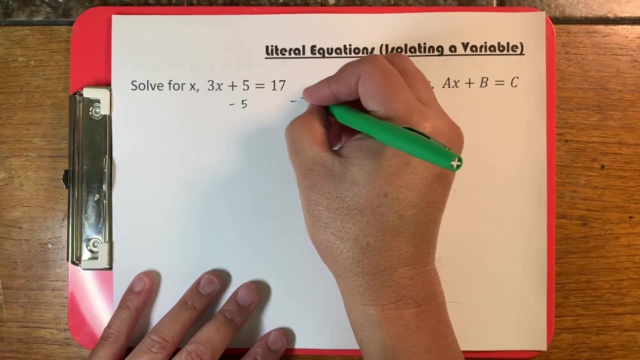 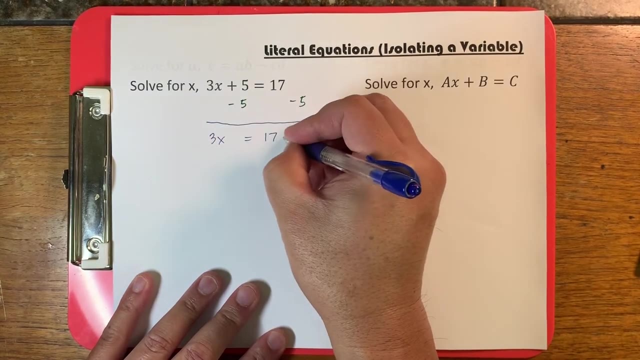 Something like this over here on the left side: If I were to ask you to do this, the first thing you would do is: well, let me get rid of that five. So you subtract five from both sides And we get three. x is equal to 17 minus five. And then, just for this example, 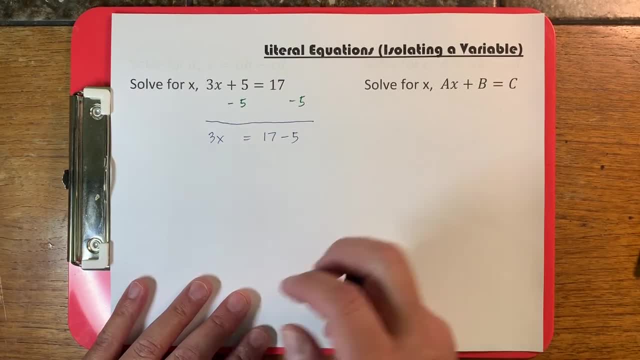 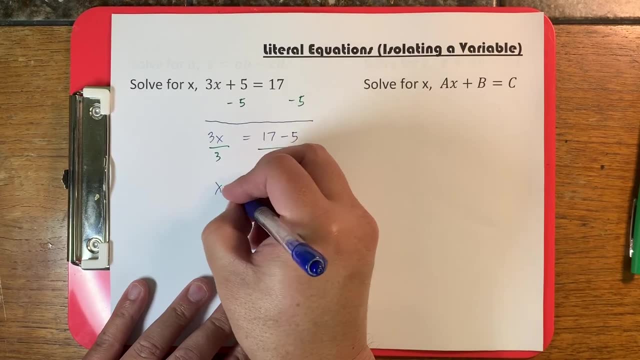 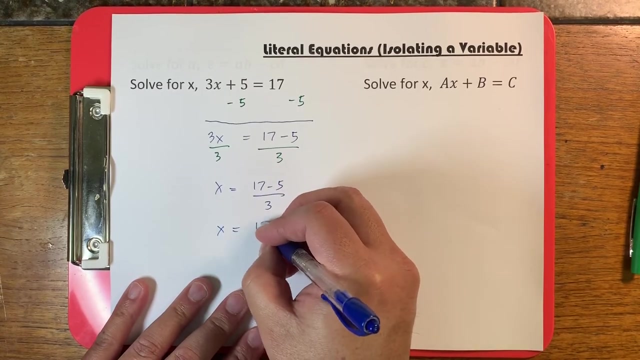 we're not going to actually do the subtraction. We're now going to divide both sides by the three, And then I would get: x is equal to 17 minus five divided by three. And if you were to sort of finish up this problem, you would get 12 divided by three and x is equal to four. 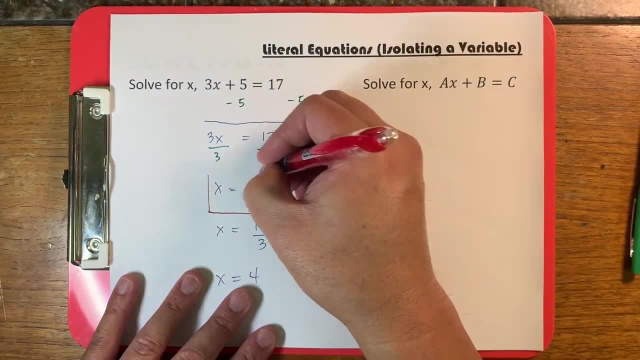 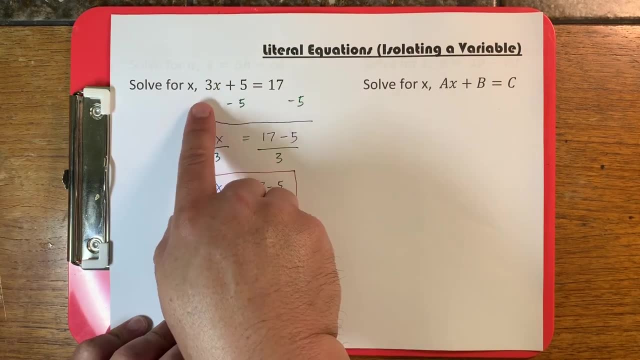 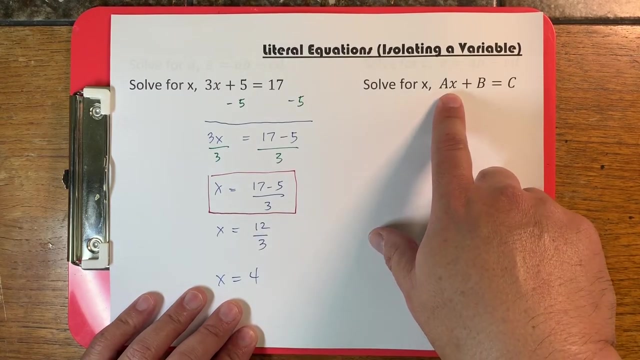 What we're going to do is we want to focus on, to what we have over here. So, in order to isolate the x, what we did was contract the five and divide by three, and that's what we have over here. Now we're going to do the same thing over here. What I want to do is I want to isolate this x. 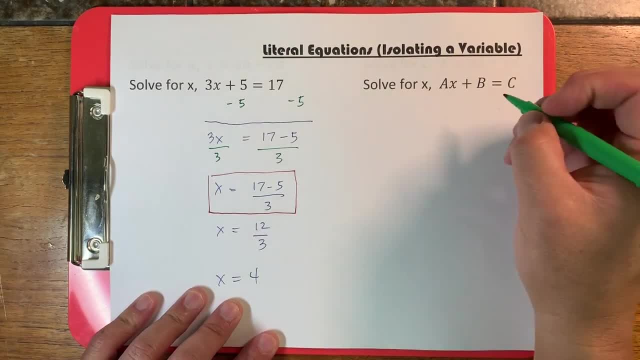 So first thing I want to do is subtract the b. So I'm going to subtract b here And I'll get: Ax is equal to seven. So if we subtract the b and we check that the answer is B, Then subtract the b and we get the sum of the contths.